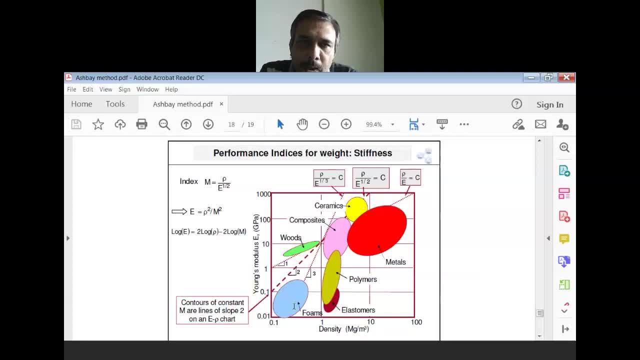 of log of M will get. slope of this line will be 3 and for that, if you plot, the materials will be, it will be getting some grades of foams and some grades of exact tangent to composites. okay, so if you don't file it as a realist material, then 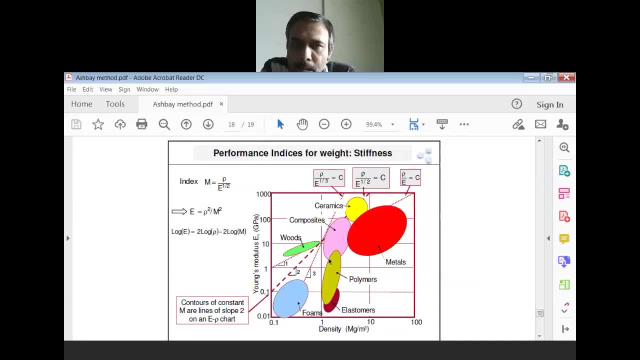 you can take that B instead of one, you can take it to two, and this line may go, may shift towards this side, towards composites and ceramics side, and you can get the appropriate grades of material. so likewise, you can work upon the performance index. once the performance index is worked upon, then you can choose. 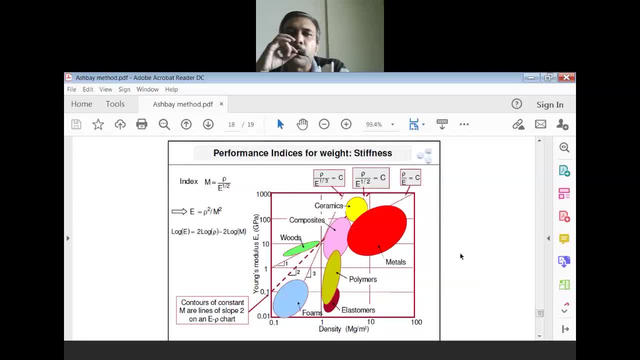 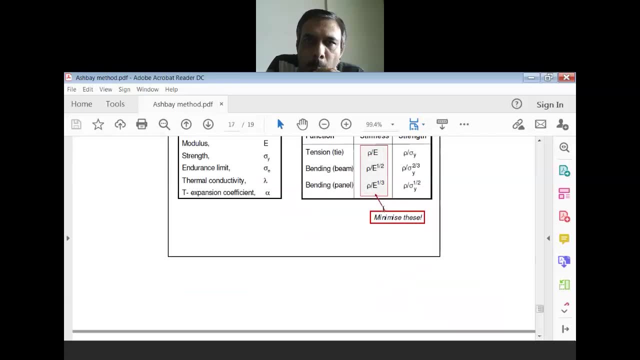 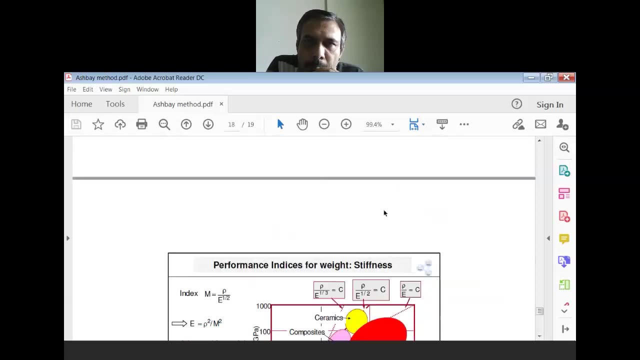 the appropriate Ashbae chart looking towards. what are the parameters you get in the performance index, as in this, all the three performance indexes. you had got the parameter as Rho upon E, so Ashbae chart selected was Rho upon E modulus, Young's modulus versus mass density. similarly, if I go it on the basis, 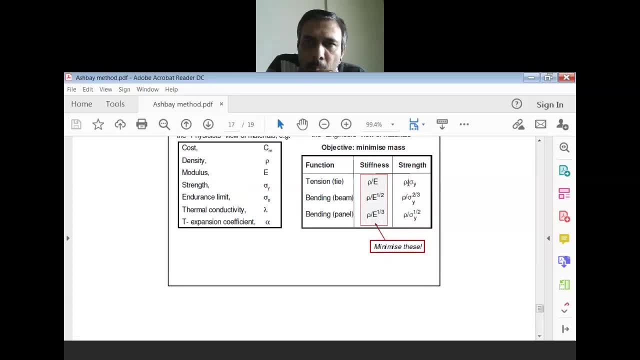 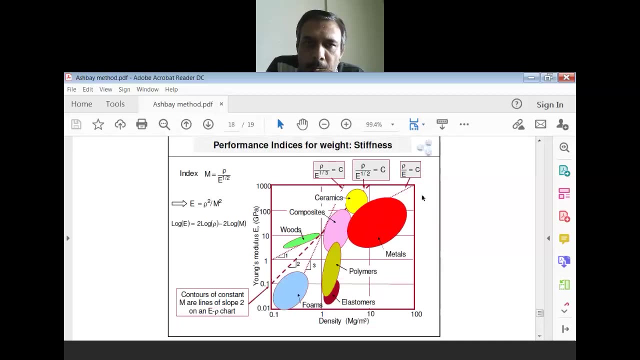 of strength. then you will find, for same light and strong tie rod, the Ashbae chart performance index. you get the parameters that are Rho upon Sigma Y, that is mass density upon yield strength, and then instead of modulus you can select a Ashbae chart which will have yield strength versus mass density, and on that chart, 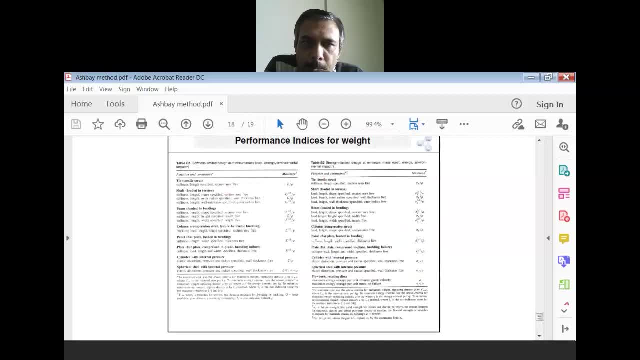 these different lines and then, accordingly, you will get the appropriate material. so if you go for this, you will find. these are the different performance indices based on the weight. if you select a tie rod, then performance index was e upon rho for sharp loaded in torsion. this: 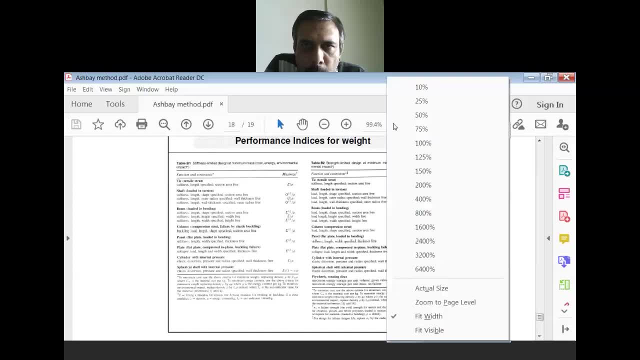 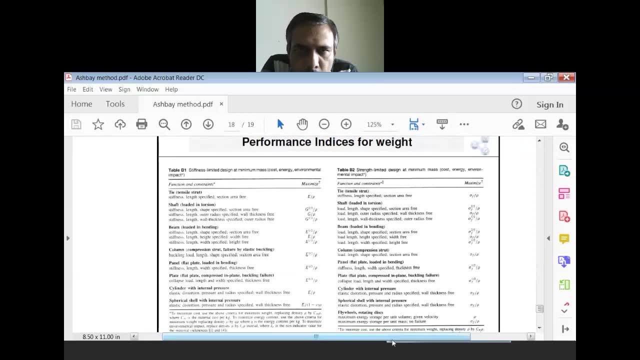 performance index comes out to be g, raised to one half upon rho. likewise, i'll just zoom this so you can see it. okay, so is it readable? now you can clearly see: for shaft loaded in torsion, in which stiffness, length and shape is specified and cross section is free, you get the performance. 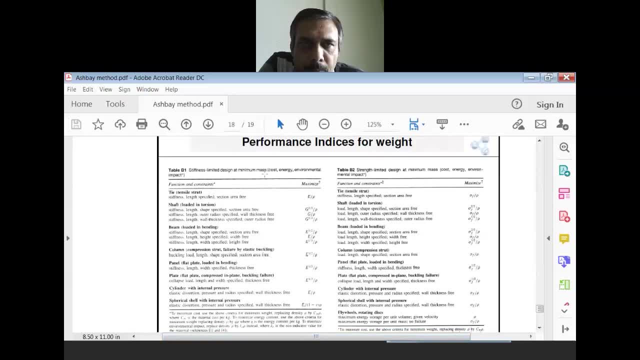 index as g, raised to one half upon rho. this side it is stiffness, limited design. with minimum mass either. the objective function can be cost, energy, environmental impact. likewise, and on right hand side of this table you have that is strength, limited design. on left hand side, that is stiffness, limited design. and on right hand, 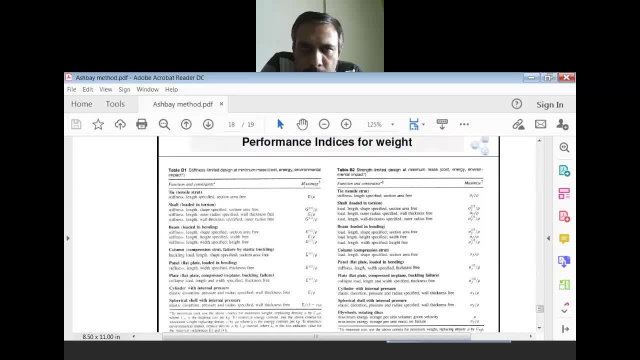 side you have strength, limited design and for different components or for different function elements, you will find you get this performance indexes, this, if you want, you can derive also for that appropriate applications and then you can reach up to this performance index. or likewise, you have table also available. you simply identify what is the component and what is your objective. 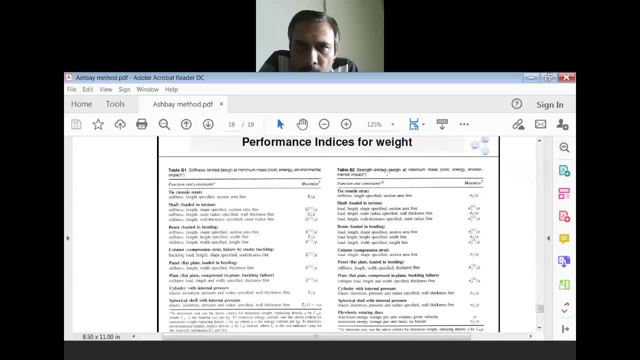 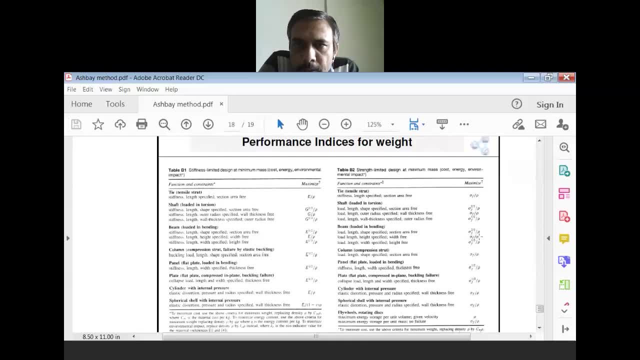 section is free. you get performance index as yield strength raised to two by three upon rho if it is a flywheel with rotating disc for maximum energy storage per unit volume and given velocity. you get performance index as mass density to minimize that for minimum weight of flywheel. you can minimize the mass density for maximum weight of. 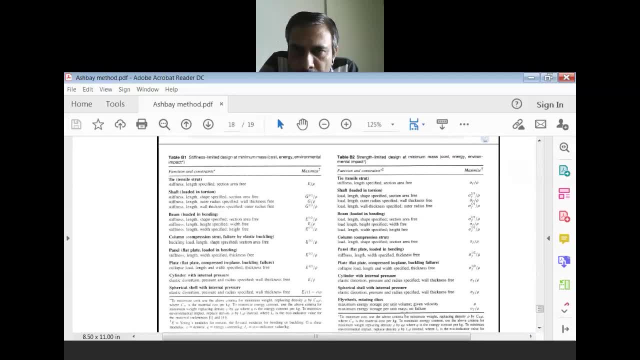 flywheel you can maximize the mass density. second objective function for flywheel was maximum energy storage per unit mass with no failure strength basis performance index of sigma F by sigma Y upon rho. so you can maximize this energy storage by maximizing this performance index is sigma y upon rho. So accordingly you can choose appropriate function or appropriate component. 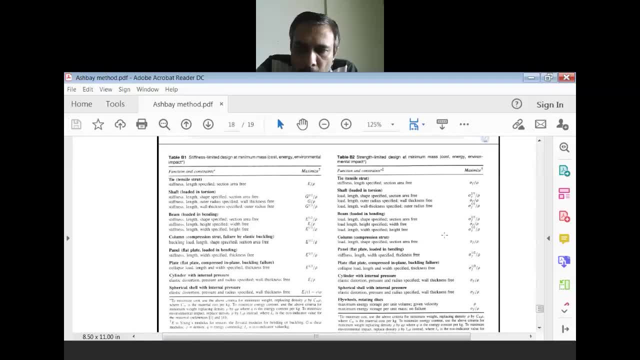 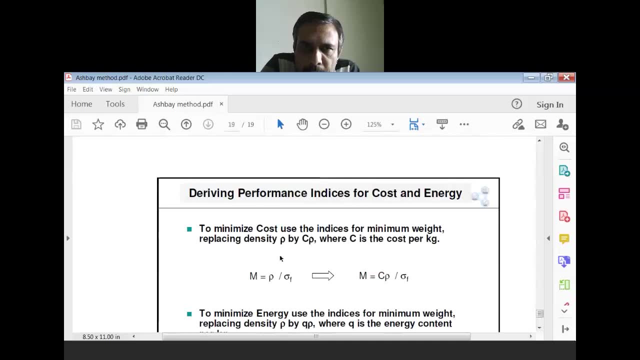 where it lies in that, and then you will have a performance index for that and this performance index is plotted on HB chart to select the appropriate material. So other if you go on the basis of cost and energy, you will find only this parameter performance index on the basis of. 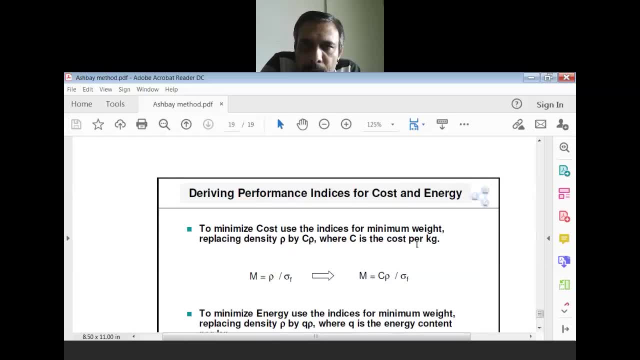 minimum mass it was rho. upon CF you will find rho will be placed by CP where CP is what CP is cost per kg. sorry, C into rho. upon sigma F, where C is cost per kg, rho is mass density and sigma F is the failure strength, that is, yield strength. So if you want to account for cost also, 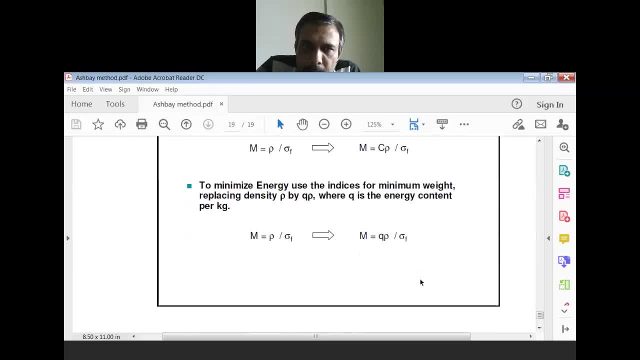 in the performance index cost parameter can be accounted. if you want to go for maximizing the energy parameter, Then you will find one more term will come in this performance index that will be M, will be equal to rho, Q into rho upon sigma F, where Q is energy content per kg, and so that can be the performance. 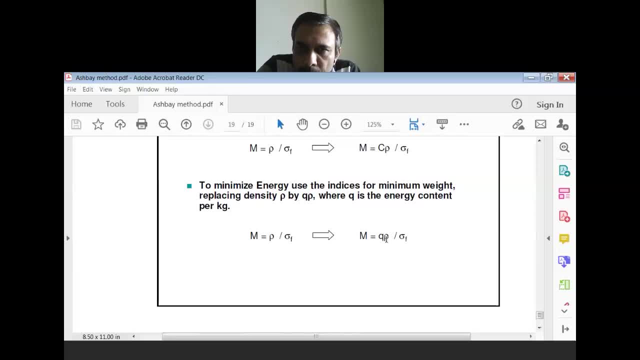 index and accordingly you can select this. So it becomes a multi variable parameter. but in this you select the HB chart of rho upon sigma F, sigma Y, and then, once you find out that candidate materials, then you compare that candidate materials which will have maximum value of Q, and then accordingly that will be the appropriate material. On above case, again you have 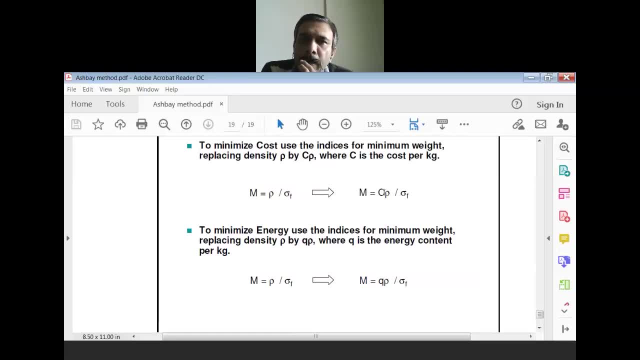 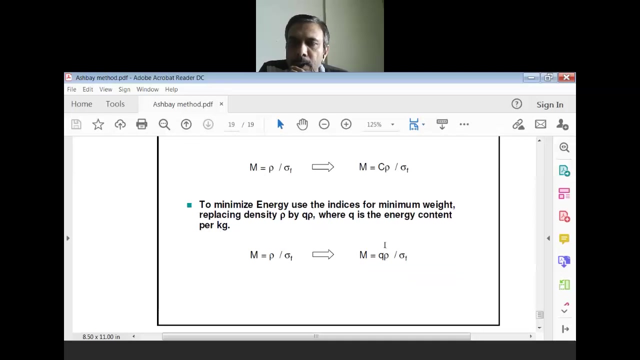 to plot graph of rho upon sigma F or rho versus sigma Y and you select the candidate materials and compare that on the basis of cost per kg. which material will have minimum cost per kg, that will be the most appropriate material. So this is the multi variable aspect. using HB technique, Instead of one variable I can go for two. 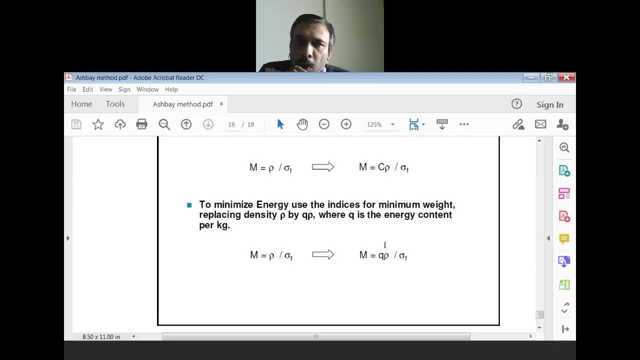 simultaneous variable, that is, minimizing the mass of the component simultaneously, it will have maximum strength and minimum cost. or minimizing the mass of component with maximum strength and maximum energy transmission. So this is multi variable problem. Okay, so likewise you can work upon. Now we'll see how to solve this problem. 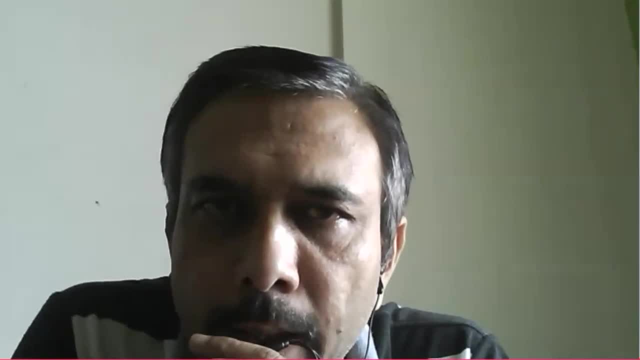 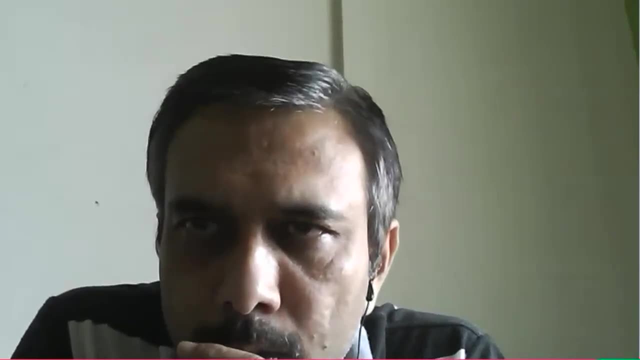 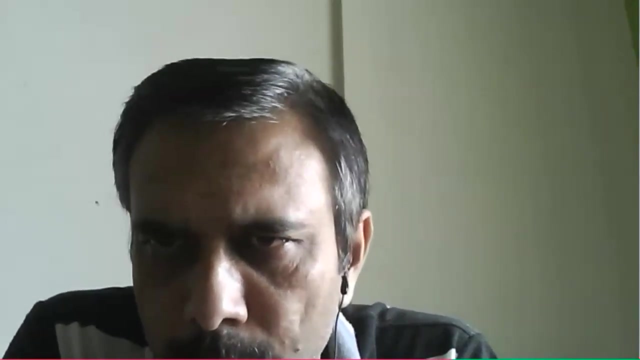 Now we'll see how to solve this problem. So we'll see upon. that is some examples for this we'll discuss now. Is it clear with this? any doubt regarding this? Yes, any doubts regarding HB technique? how to select it? Yes, any doubts? 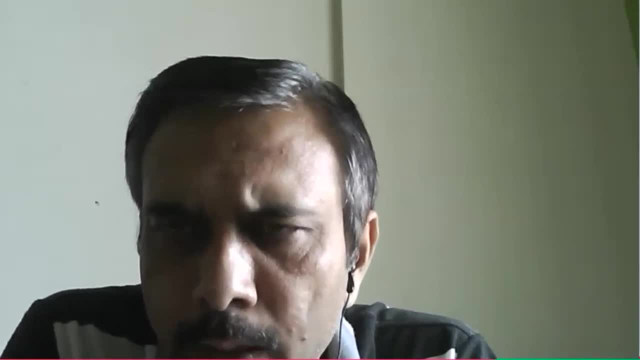 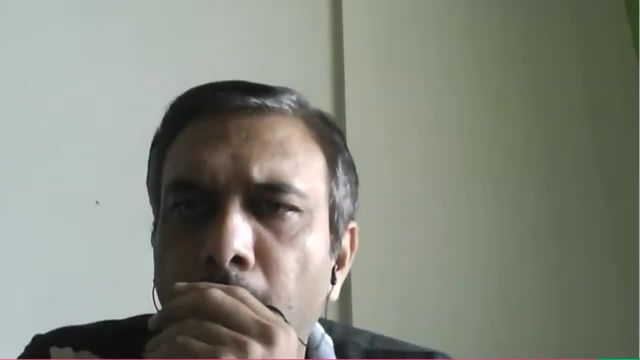 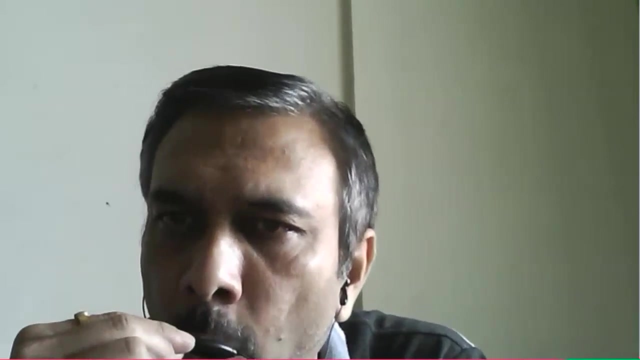 Okay, there are some doubts asked in the chat box How the power of E is decided in expression. It is not decided. you had got that from deriving the performance index. You had derived the performance index and in that you had got the value of E. it was for. 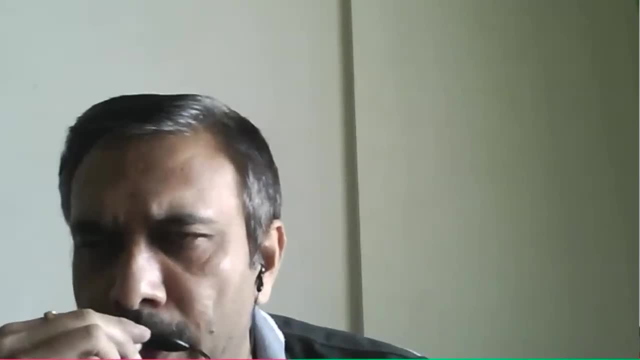 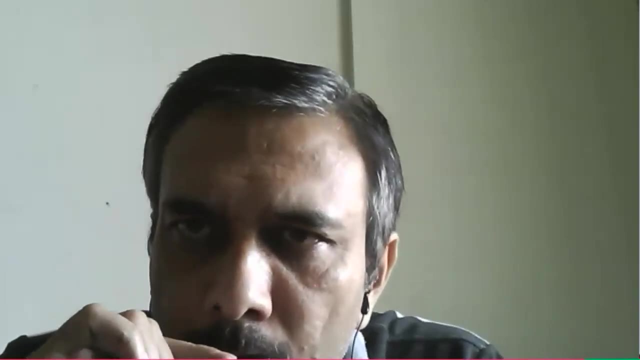 stiffness based design. it was rho upon E. we had got as a performance index. So we are. Amol is asking something. now what is what is that exactly? what do you want to ask? It's not very much clear. Yes, Amol is here. Amol. 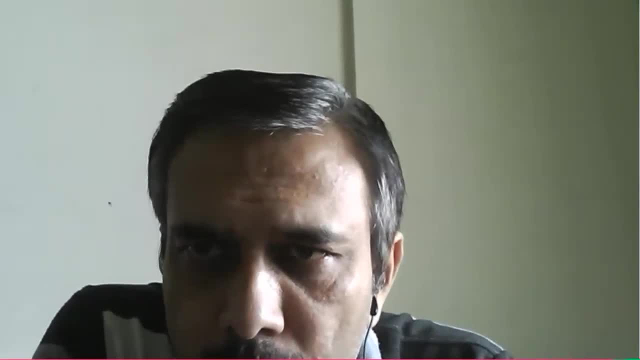 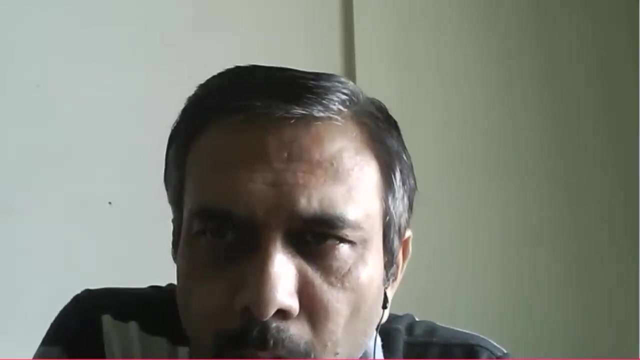 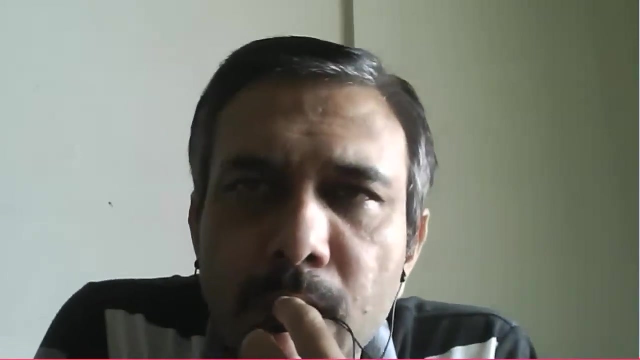 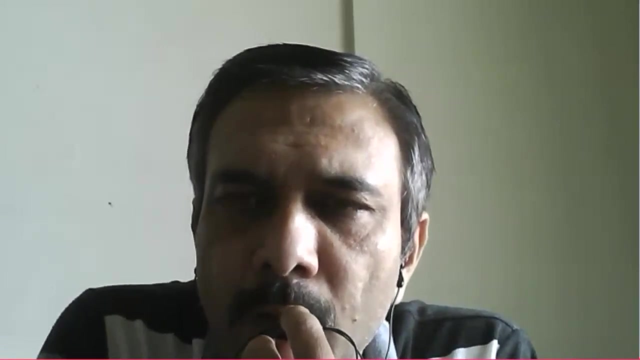 Amol, Amol, Amol, Amol, Amol, Amol. can you hear me? Amol, Hello, hello, hello. can you hear me? Hello, hello, hello. Hmm, what's that? Amol, is there, Amol, Can you hear me? 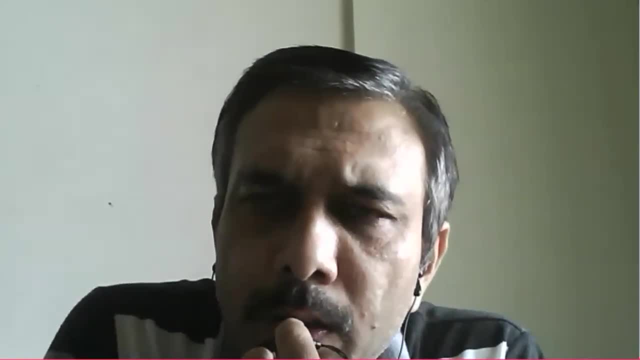 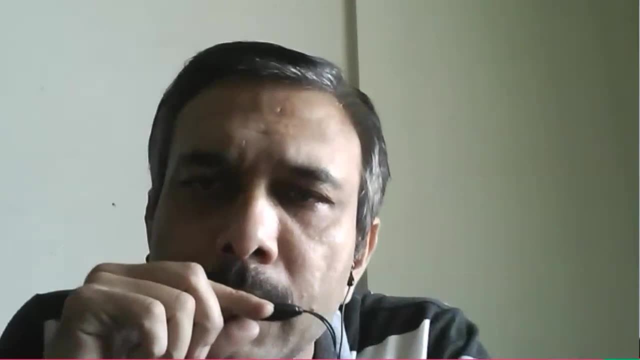 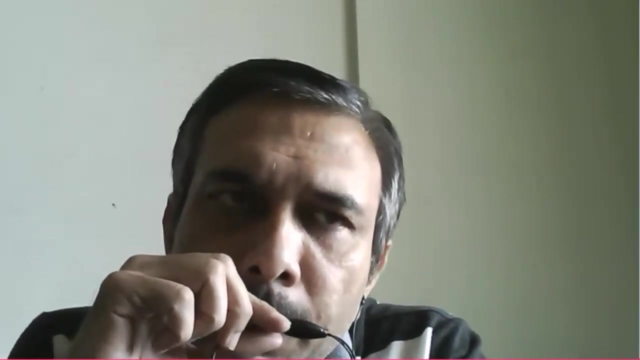 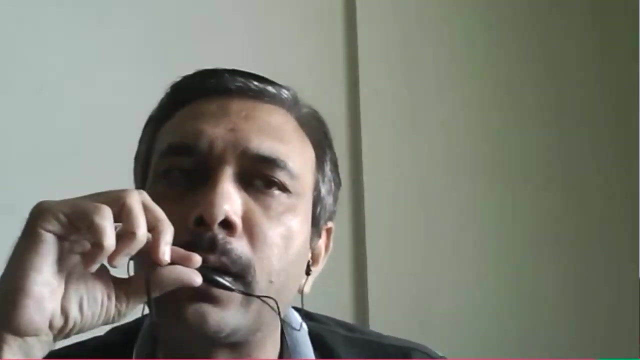 Amol. So okay, what he is asking is how the power E is decided in expression. You need not have to decide it in the expression It is. you have to draw a graph of E versus. you have a graph of E versus density and then where the line cuts that graph, the material lying nearby that line will be that particular candidate materials. 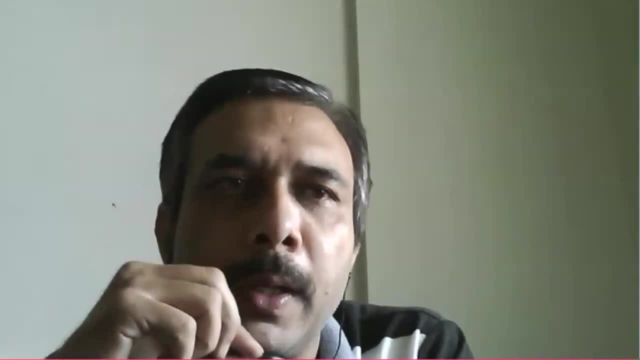 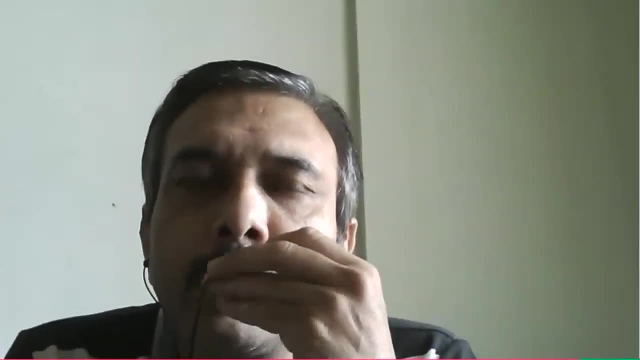 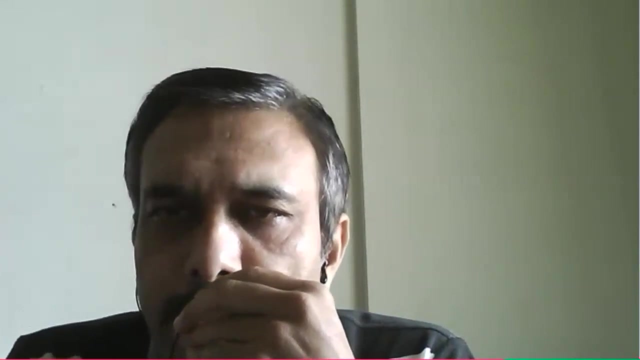 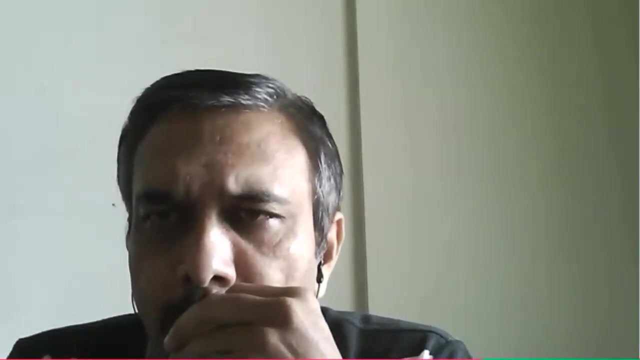 Now for this candidate material. you work out this ratio of rho upon E. for each and every candidate material you will have the value of E available for material property chart as well as the value of rho will be available to you and then, accordingly, you select that material which will have minimum value of rho upon E. Is it clear? Okay, So he has written. it is understood, Okay, fine. Second question: it is: is the power of factors like 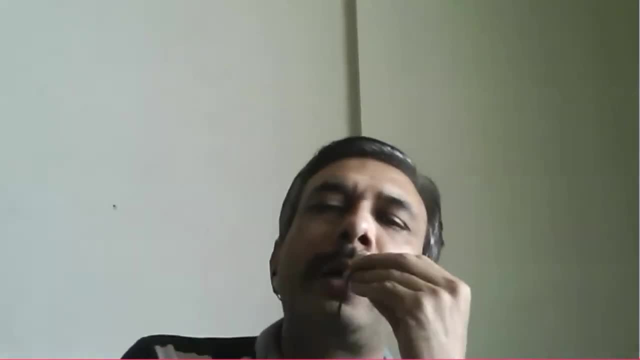 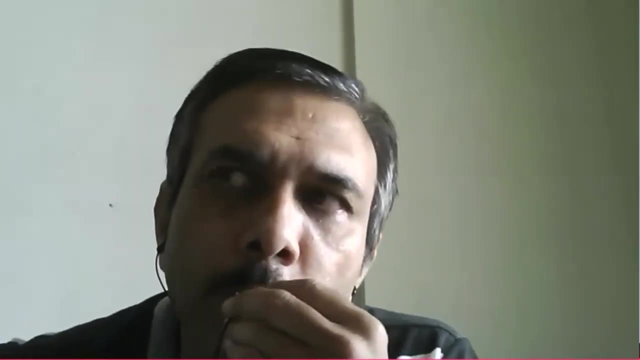 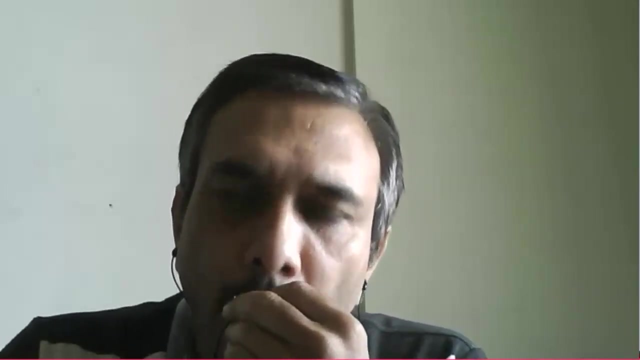 cost and energy. always one. No, nothing like that. How could be? the factors will be one always. Once you reach to that equation, Y equal to AX plus B, then we can assume the value of B as one or two. You have to, as you go on, assuming that if I go for one, what is the value of M you are getting? then? plot that line over there. Then, whether it is cutting the appropriate materials or not, that you have to see. Okay, fine, If it is cutting the 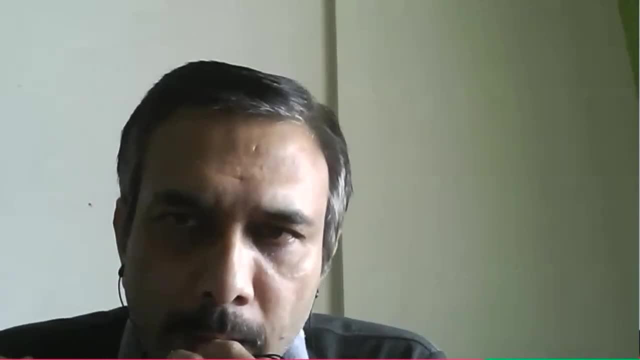 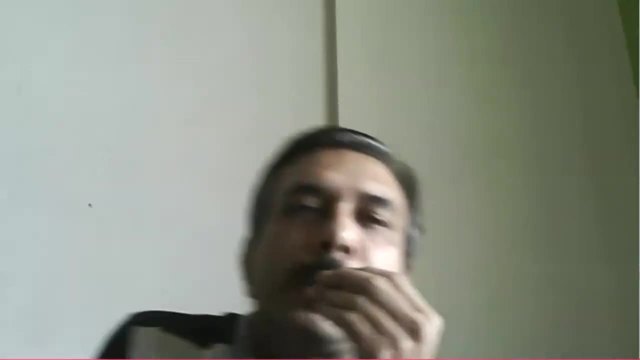 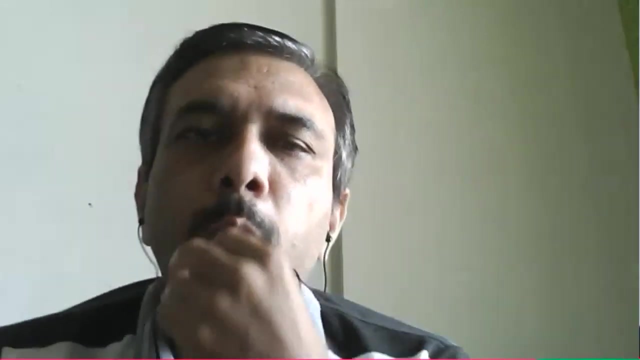 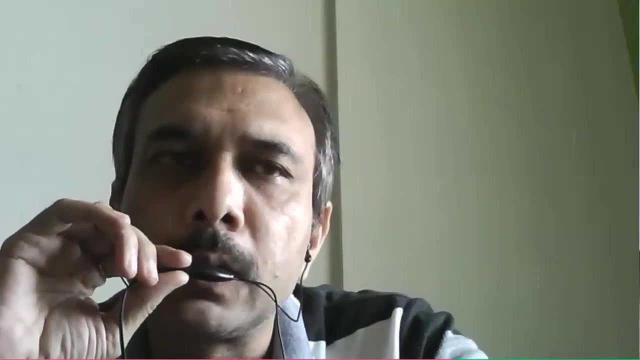 value of M, then you can keep it, or else you go on increasing. now, instead of one, I'll take B- value of B- as two or three and accordingly I'll plot that line over here. Okay, For the case of cost and energy, it is the value parameter which we had just now seen, that was C, C was cost per unit mass. unit cost per kg. Likewise, for energy, it was Q- Q was energy per unit mass. 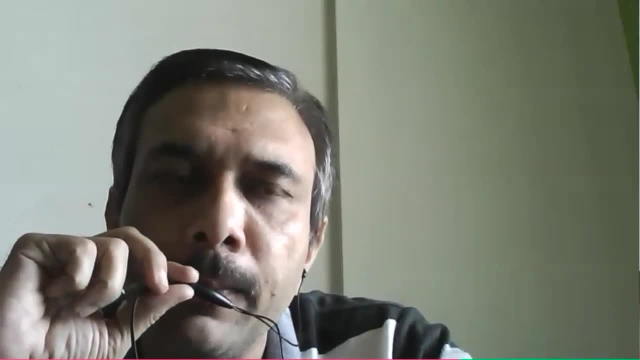 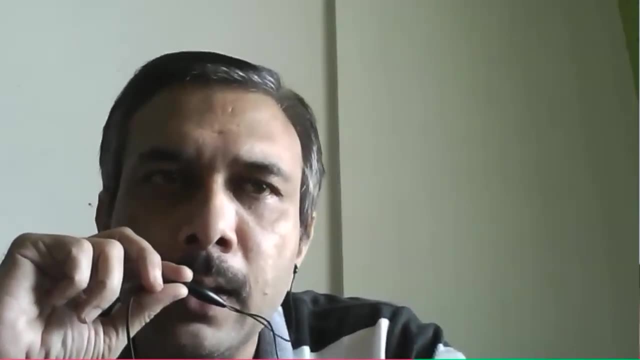 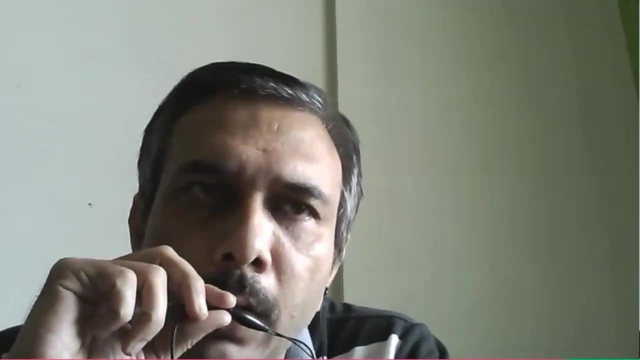 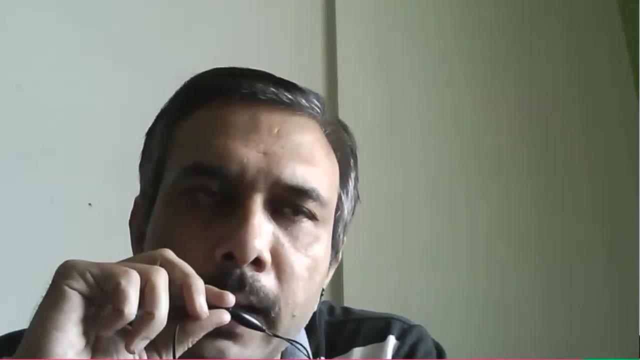 So these parameters, these values, will be available in material properties. Now, cost for rate rate of the material is known to you from the market survey, So you can work out what is the rate per kg for cast iron, or it could be for steel, whatever may be candidate materials, Then that is a multi objective. just now we had seen that example. Then plot the performance in this line on the chart of, say, rho upon E, that is, mass density and modulus. 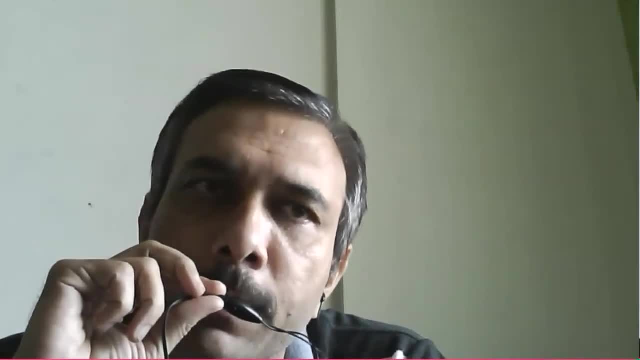 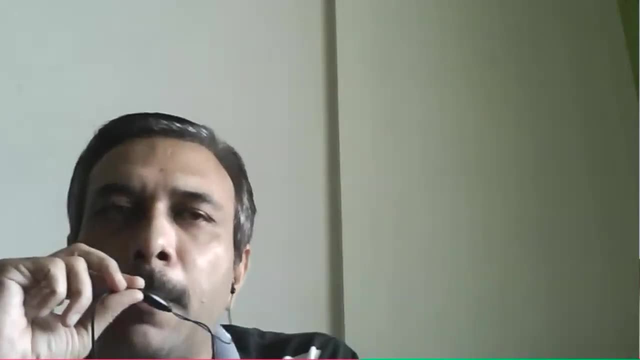 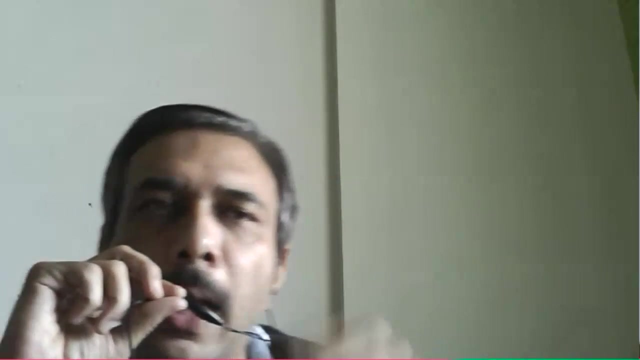 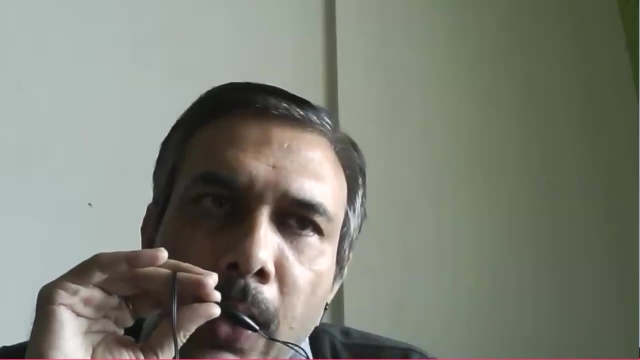 And then, once you get the candidate materials, compare that candidate materials which will have minimum rho upon V as well as which will have minimum C. that is cost per kg, So that material which gives you that product of C into rho upon E, this product you have to work out, and the product which minimum C into rho upon E will be the most appropriate material which will have that objective of C into rho upon E. 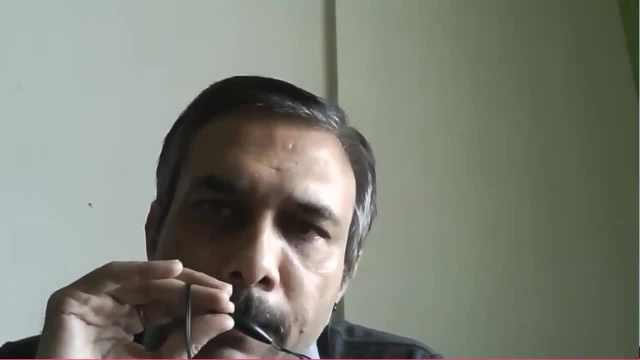 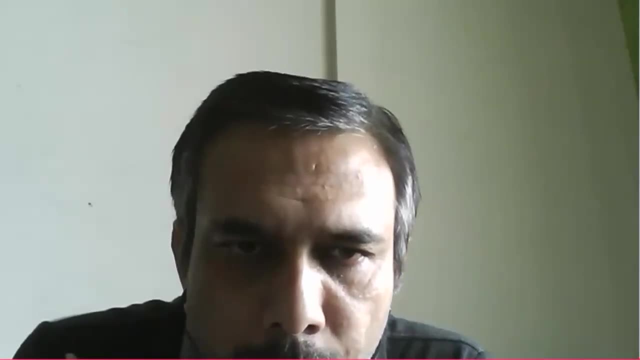 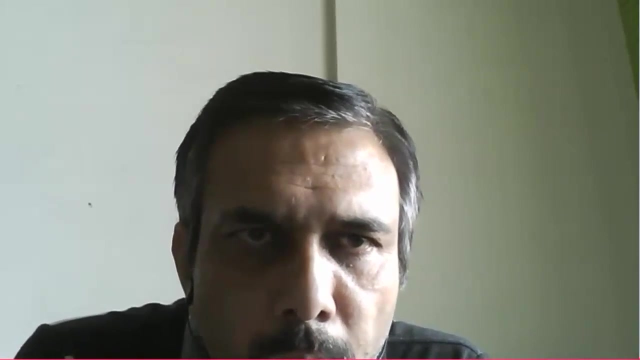 So light and strong tie rod or light and strong beam with minimum cost. Clear with this, because performance index came was rho into C upon E. Clear with this. We will see few examples and I feel you will get much more idea on that. I will just go to that next slide now So that some examples we will discuss and you will get more idea on this. 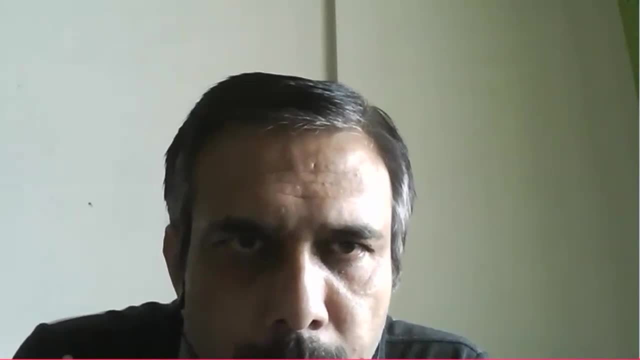 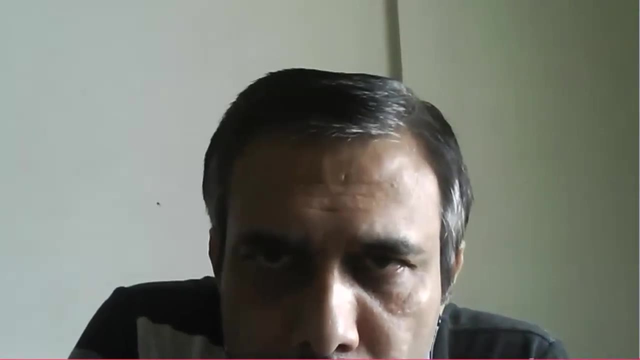 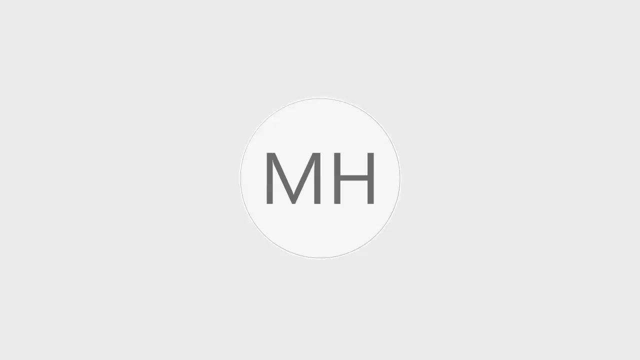 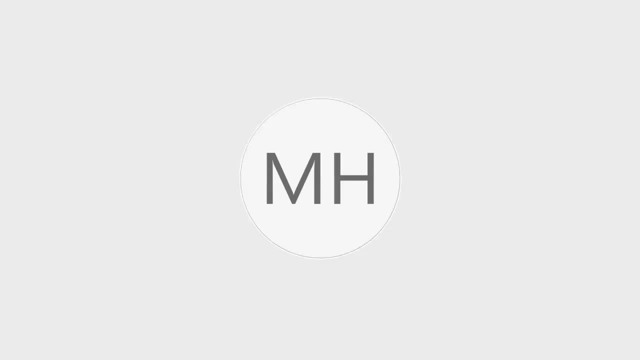 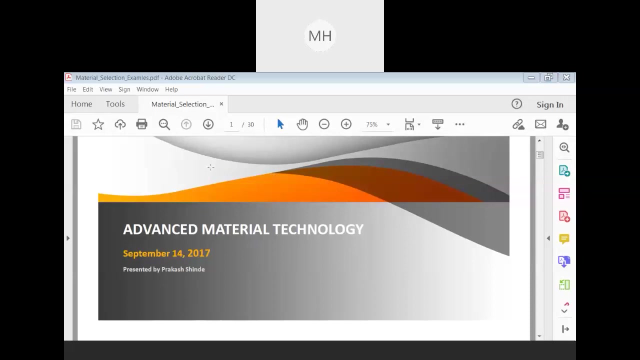 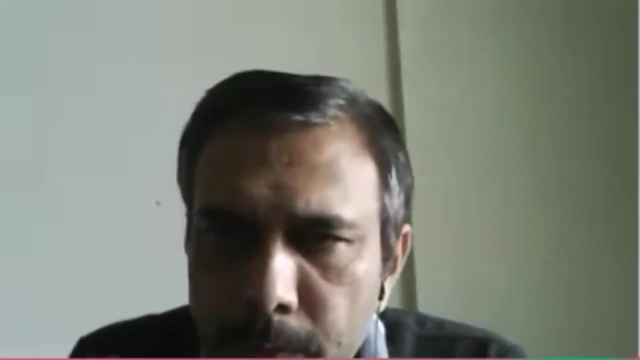 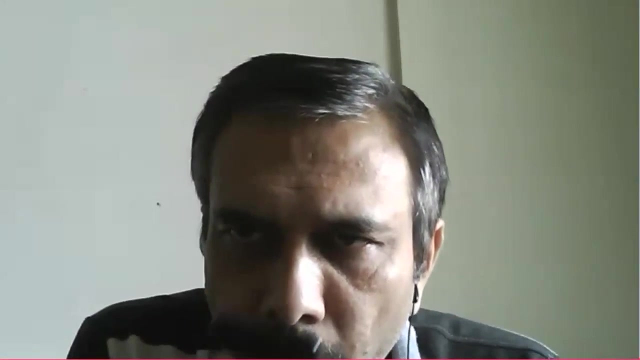 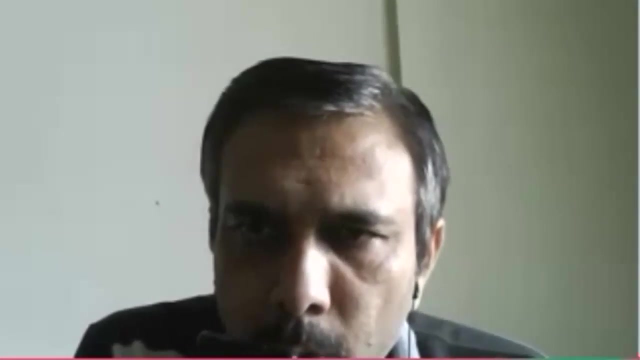 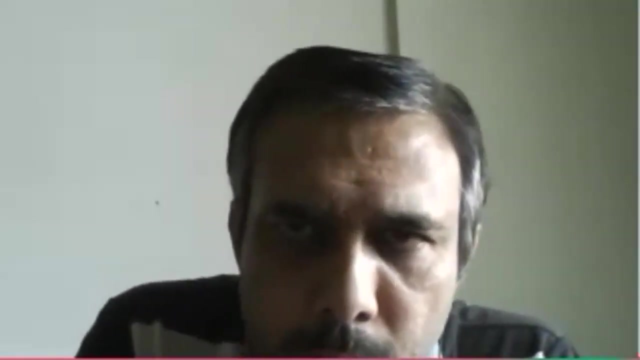 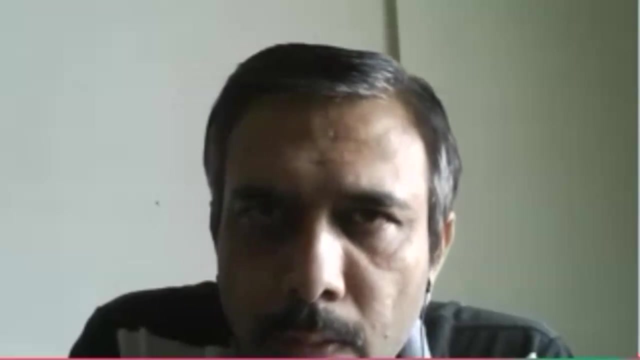 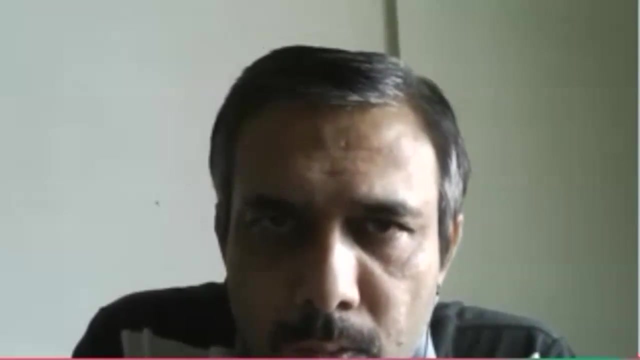 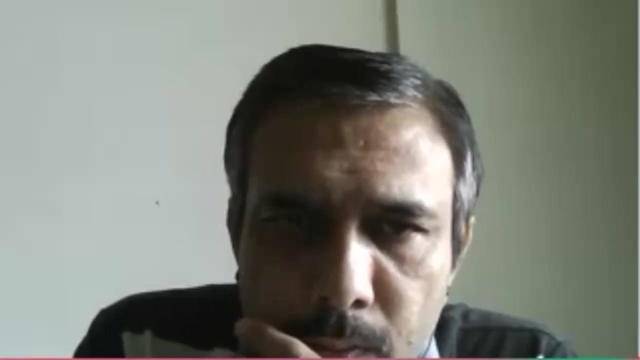 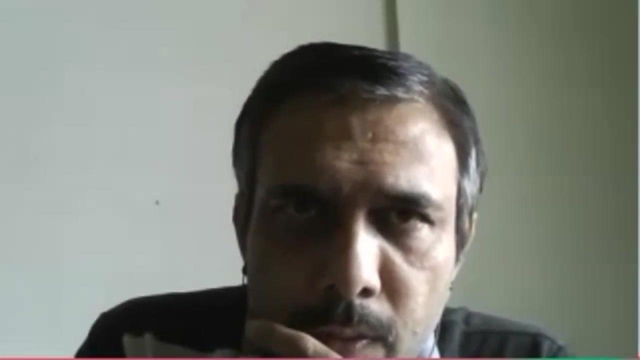 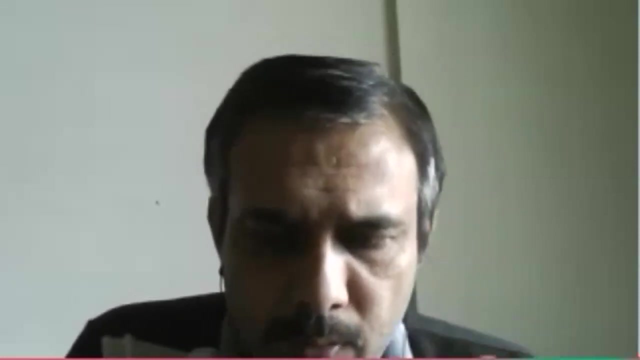 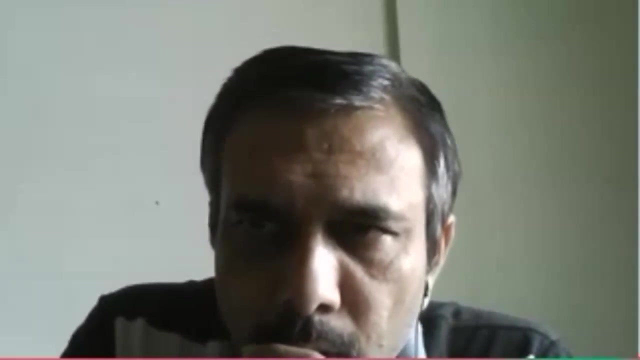 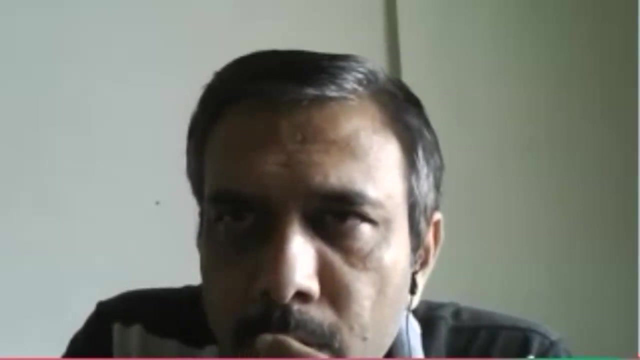 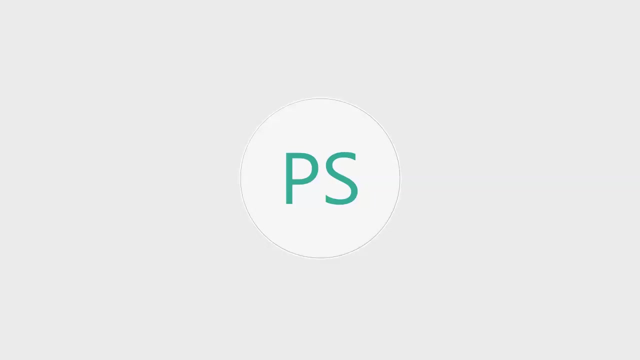